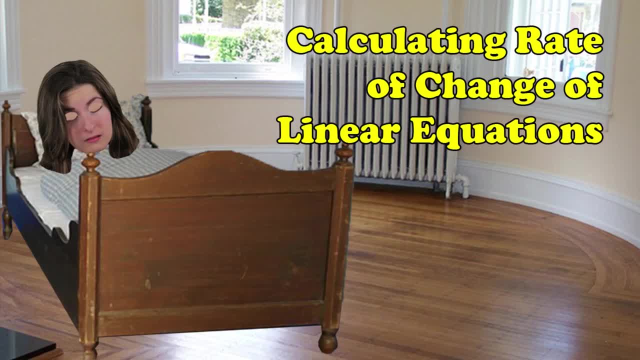 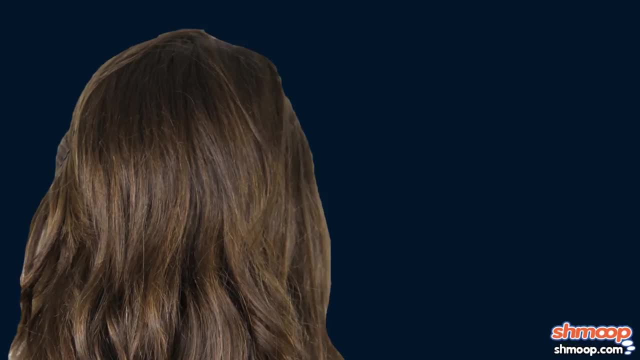 Calculating Rate of Change of Linear Equations. a la Shmoop Shoot. you're running late for school again. Why did you think it was such a good idea to play Candy Crush till 1 o'clock this morning? You can't dwell on it too much. 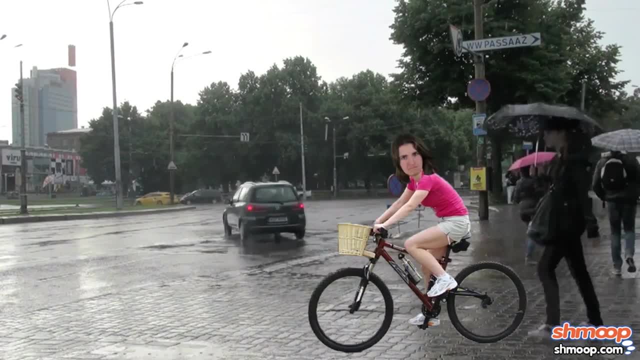 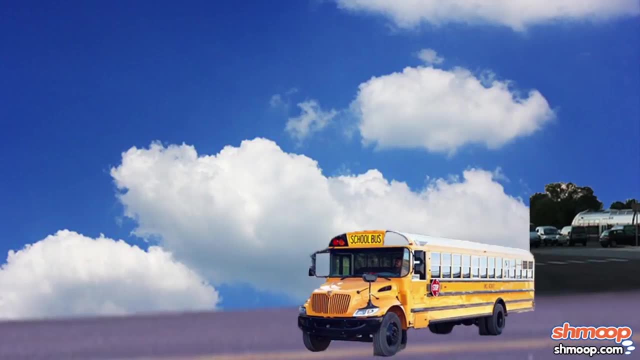 You have to make the bus or you're going to have to bike to school in the rain. Jimmy texts you at 7.34 saying the bus just picked him up. The bus left the station at 7.30, and Jimmy's two miles from the bus stop. 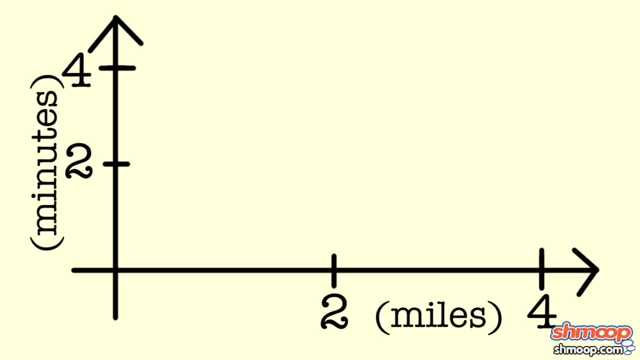 Oh boy. Well, if we were to graph the bus's path, it left the station at zero minutes and was zero miles from the station, which makes the point right here at zero zero. Jimmy's house is two miles from the station and it took the bus four minutes to get to. 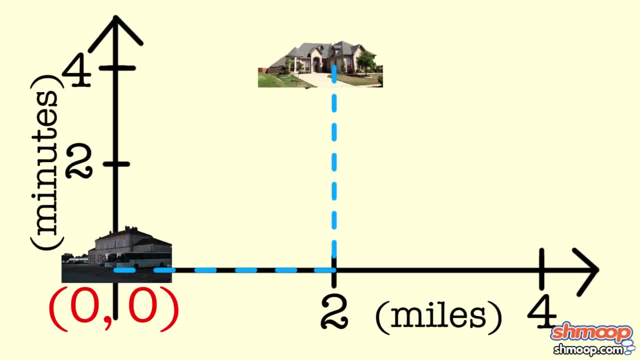 Jimmy's house, and that makes the point right here. One, two, and then one, two, three, four. Well, how fast did the bus drive from the station to Jimmy's? Well, yeah, it took him four minutes, but how fast was he going? 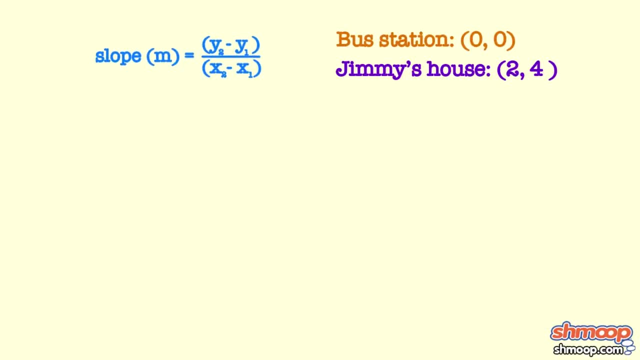 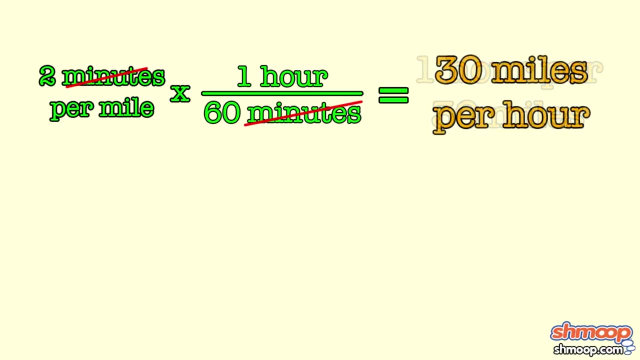 To find out, we use the formula for slope and plug in our coordinates Like this: So now we know the bus drives at a constant rate of two minutes per mile. So that's 30 miles per hour on a residential street. Well, the wheels on the bus are no longer going round and round. 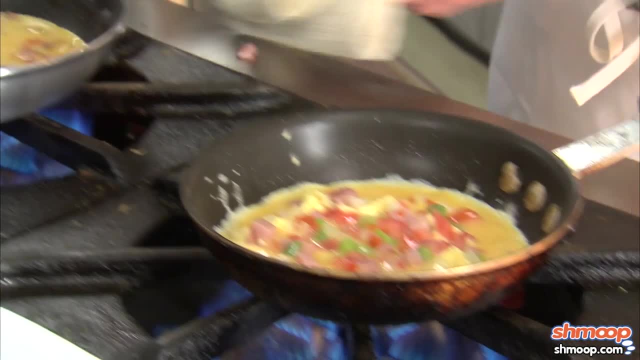 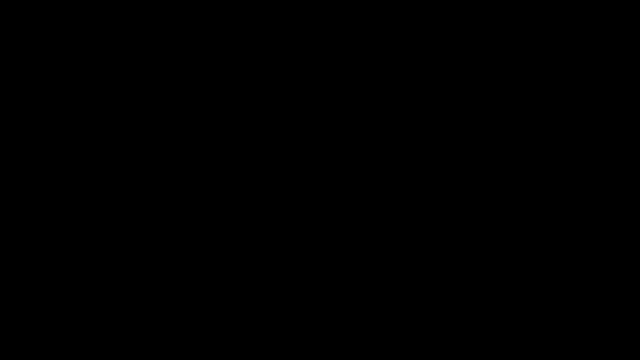 Well, we guess this buys you a few more minutes before the bus makes it to your next stop and you can make some eggs for breakfast or get a few more minutes of sleep, and there will always be eggs. What did the buffalo say to his son as he left for school? 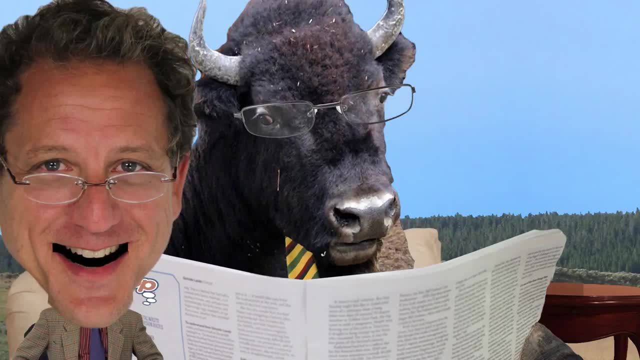 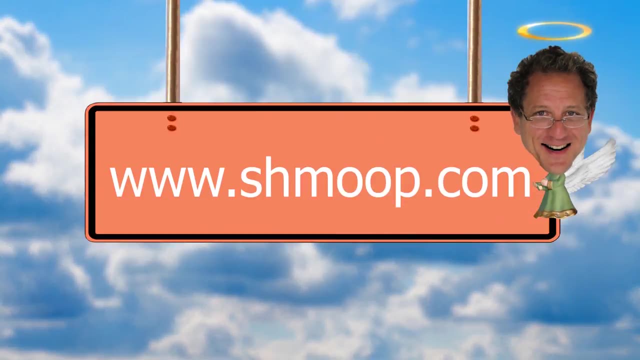 Bye son. Okay, bad joke, But if you survived it, how about clicking the subscribe button below? And if you're looking for more jokes from yours truly, why not check out our website at wwwshmoopcom? And if you want to get updates on what's new, well, check us out on Facebook and Twitter. 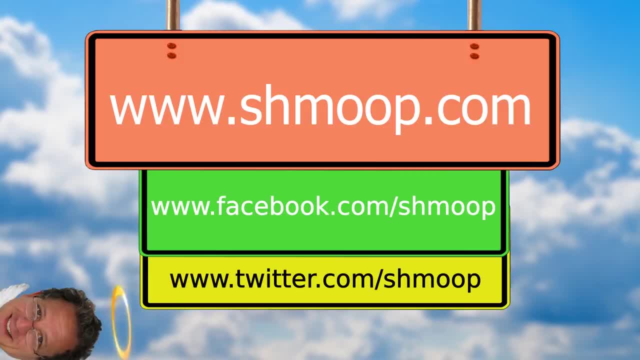 too. Please check our Facebook and Twitter pages Please.